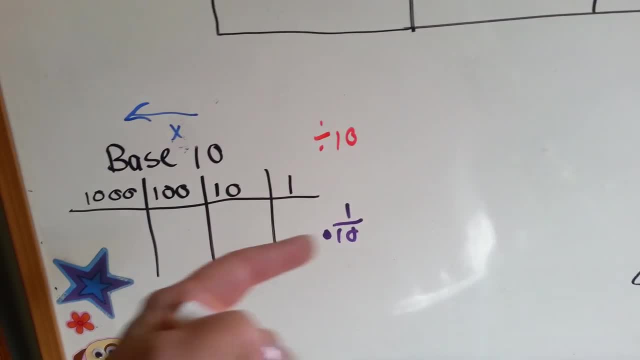 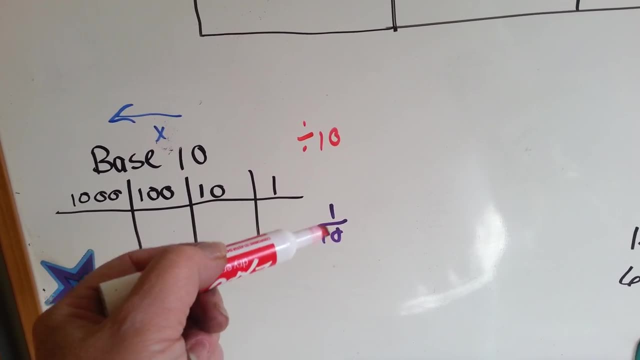 When we go this way, we divide by 10 on this side of the decimal point, on the right side, So that would be 1 tenth, 1 tenth, 1 tenth divided by 10 would be 1 one-hundredth, and we just keep going that way. So that's multiplying, that's dividing, okay. 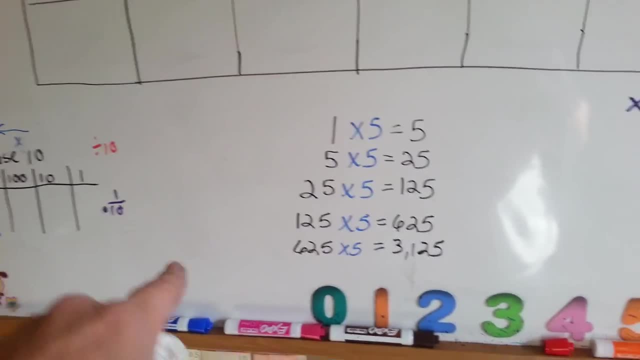 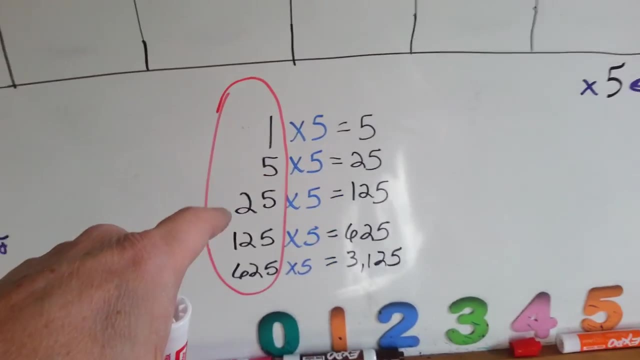 Well, in base 5, we multiply by 5 instead of by 10.. So this would be our columns for our place value: 1s, 5s, 25s, 125s, 625s. That's what our columns would look like, see. 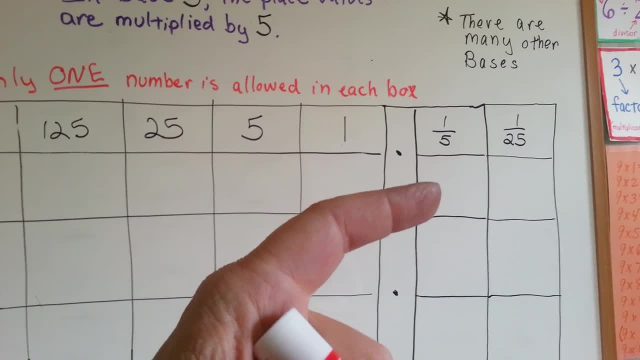 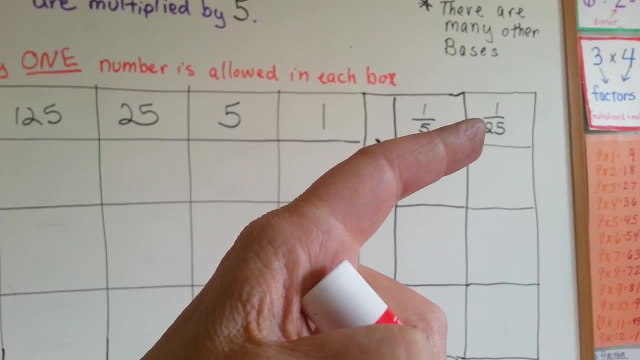 And to the right of the decimal point, we would have, instead of 1 tenth, we'd have 1 tenth, 1 fifth, and instead of 1 one-hundredth we would have 1 twenty-fifth, and it would keep going on: 1 over 125, etc. 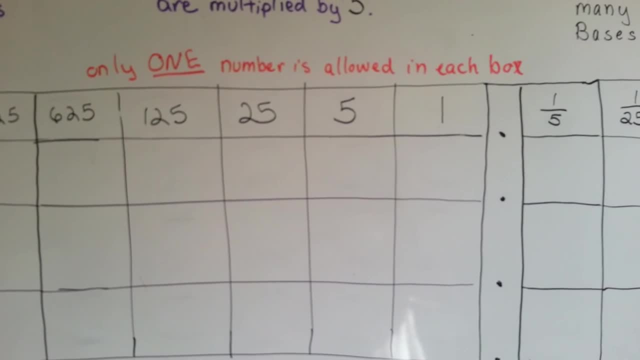 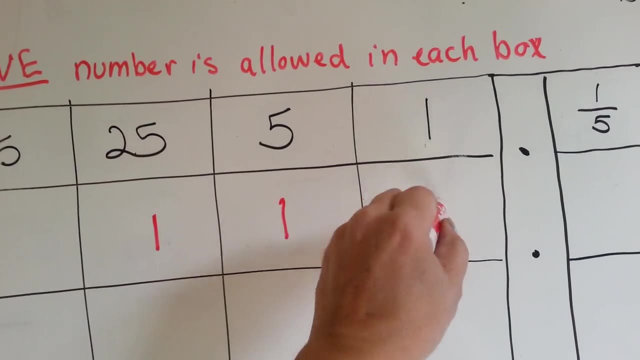 So if I wanted to tell you to write the number 30, you would have 1 twenty-five, 1 five and 0 ones. That would be the number 30 in base 10.. Kind of odd, isn't it? 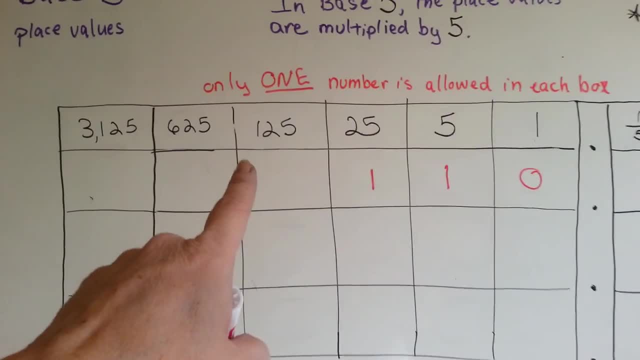 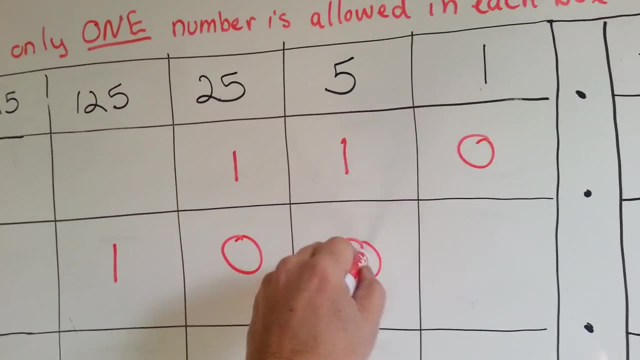 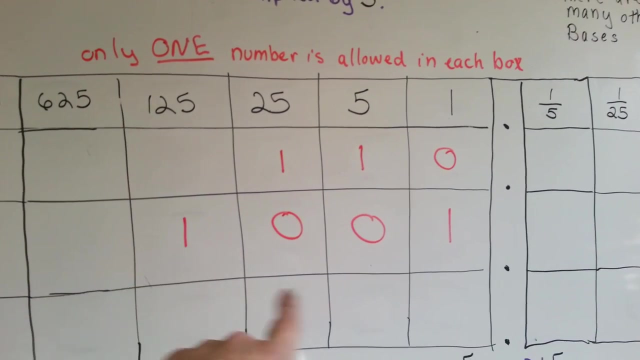 What if you wanted the number 126? You would have. If you wanted to have 1 of the 125s. you'd have no 25s, no 5s and you'd have 1 one That would give you 126.. You'd have 1 of those and 1 of those to get 126. 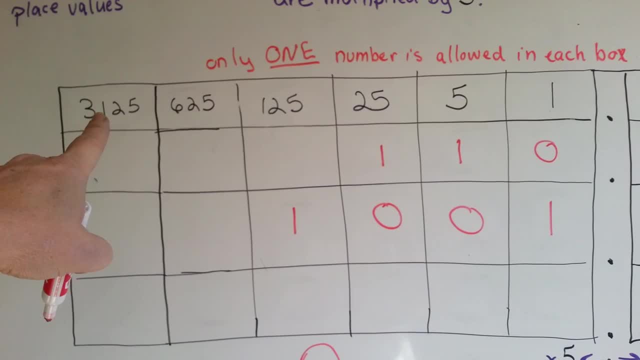 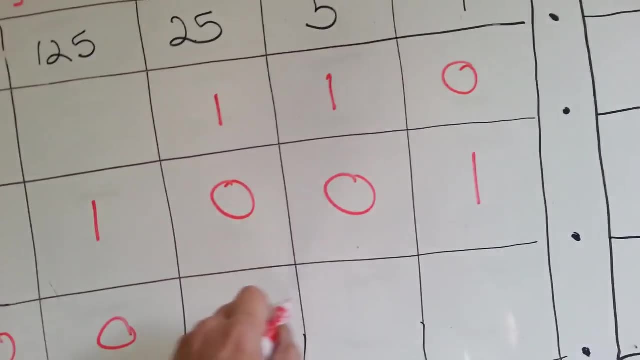 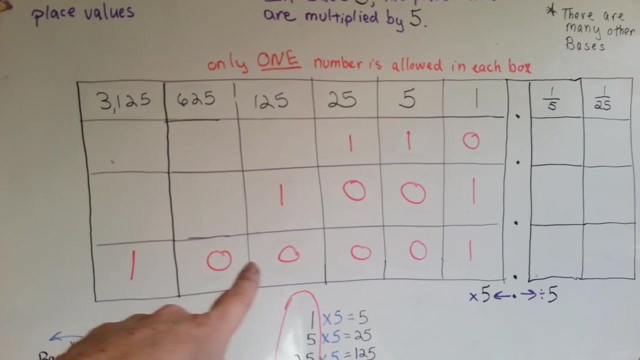 If you wanted to have 3,126, you'd have 1 of these and none of these numbers and a 1.. Let me back up so you can see That would be 3,126.. You'd have just a single 1 with 1 of those see. 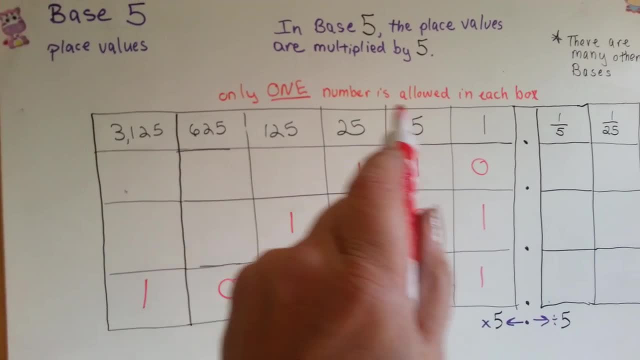 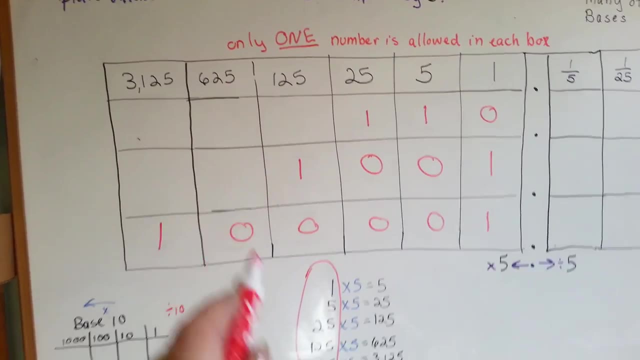 So base 5, you just keep multiplying by 5 as you go this way. 1 times 5 is 5, 5 times 5 is 25,. 25 times 5 is 125, times 5 is 625, see. 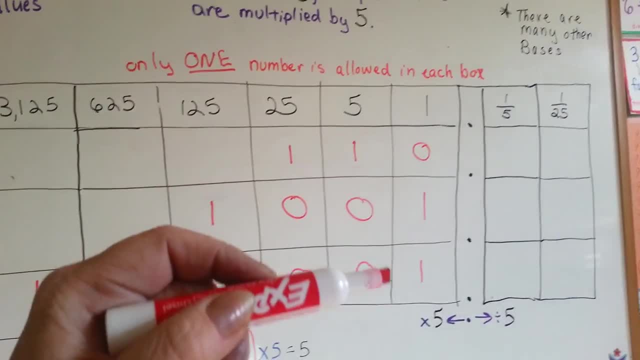 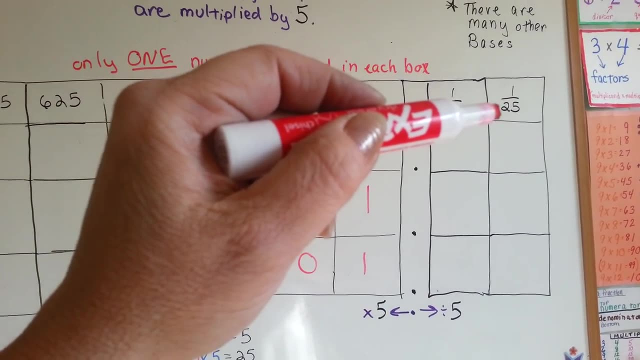 And you just keep going to the left, multiplying by 5.. And on the right side of the decimal point you keep dividing by 5.. 1 fifth divided by 5 is 1 over 25, see Very different than our base 10..